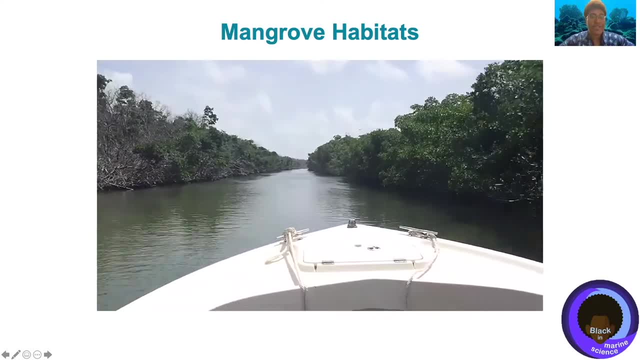 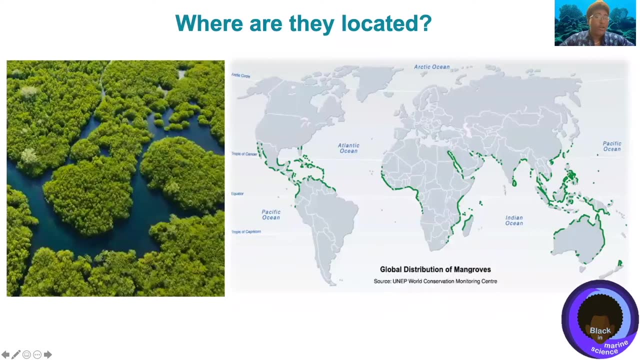 your left and your right, you'll see all this vegetation or trees. These trees are called mangroves. Mangroves are located all over the world, specifically in the hot tropical climates, and they're usually associated with coral reef environments. But what are mangroves? 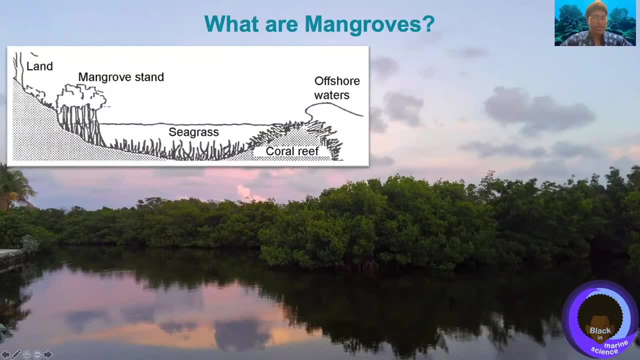 Well, mangroves, as I mentioned, are usually in those tropical areas. They're usually associated with a coral reef environment and you'll notice that the long tree system, the long roots of these mangroves, help serve a lot of purposes. For one, it prevents pollution from running off the land. 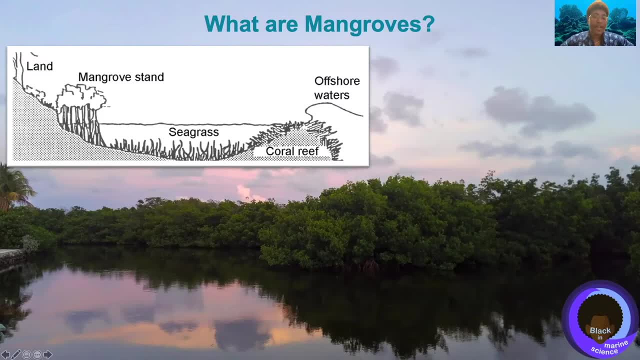 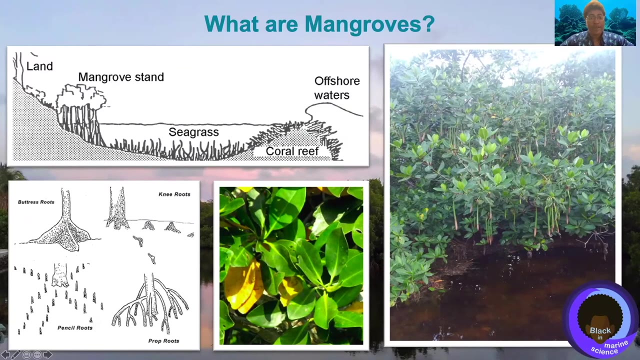 into the water and, on the flip side of that, it prevents a lot of wave action or those heavy waves from hitting the land and eroding the surface. Mangroves have a lot of cool features. They differ in species and they also differ in their roots system. They could be, have buttress roots, pencil. 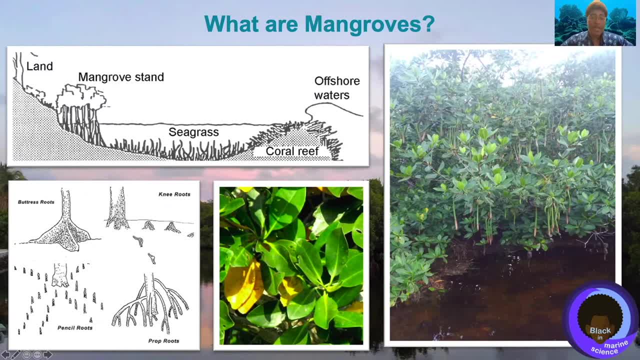 roots, knee roots or even prop roots, And all these roots help stabilize that tree or anchor it into the soil. You'll also notice that they mostly have green leaves, but they can also have yellow ones. These yellow leaves are able to store salt. These seed pods will grow nice and long they'll. 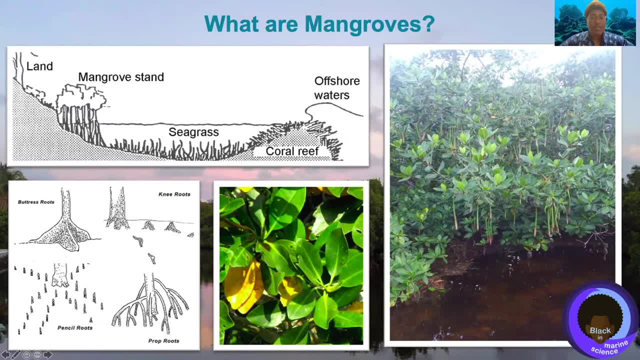 get a bit heavy and then they'll drop from the trees. Once they drop from the trees, they float in the water column, mainly at the surface, until they can find an area in which they want to lay their roots, and then they grow a whole new tree. Now these roots are super important With mangroves. 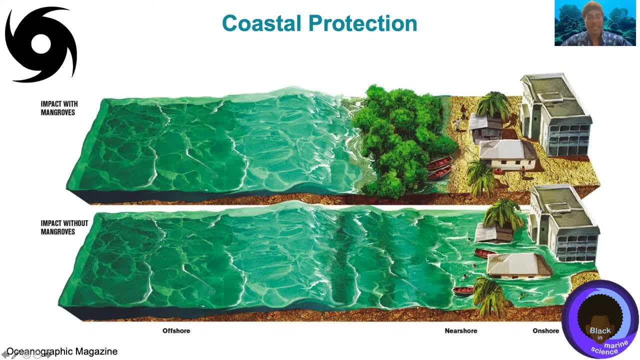 at top picture, you'll notice that when a storm comes in, hurricane or tropical storm- those mangroves prevent damage on land. but without those mangroves, those water, that water can seep into the land, seep onto shore and ruin trees, houses, boats etc.